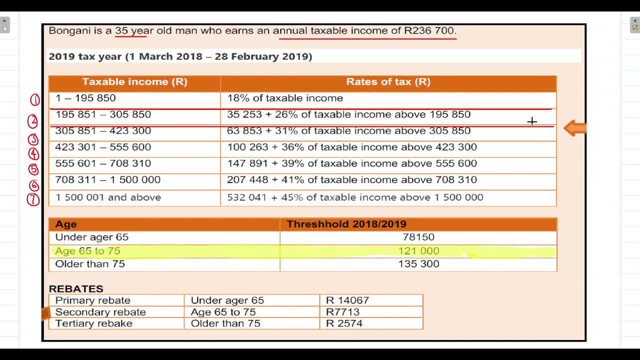 okay, So his annual taxable income falls within the second tax bracket. okay, Then, once we've basically determined that, we basically need to now find what is the total amount that Bongani earns in total taxable income. that is, above $195,850.. So we already know that for us to be able to 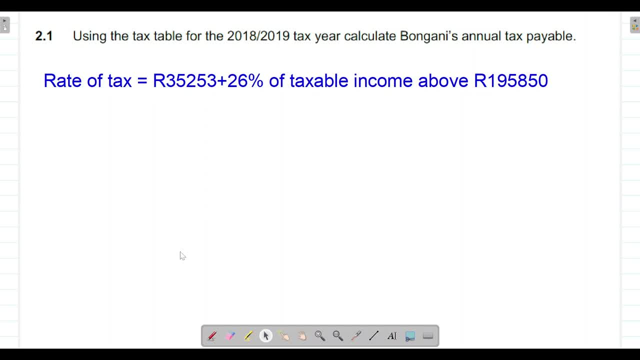 calculate his rate of tax, because we already found that his annual taxable income falls in the second bracket, right? So now what we basically need to determine now, right, The first thing we need to determine is that what is his taxable income above $195,000? So how we are going to get. 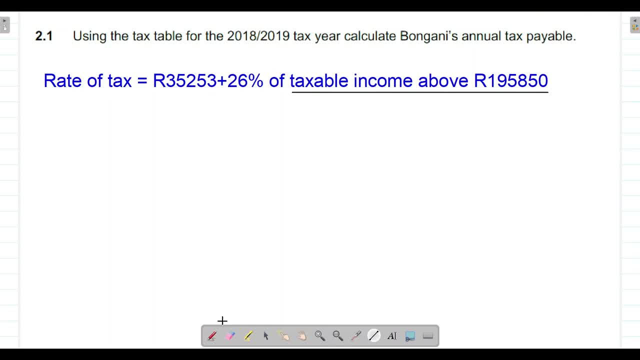 his taxable income that is above $195,850 is that we're just. you basically take his annual taxable income and you subtract that from that amount of $195,850, right? So if you do that, you'll find that his taxable income above $195,850 is actually $40,850, okay, So that is the taxable. 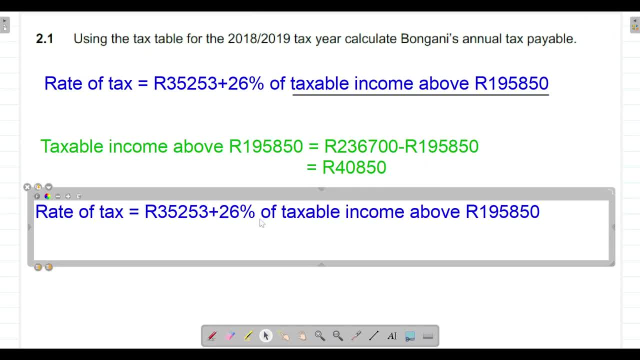 income above $195,850, okay, So since we already found what the taxable income above $195,850 is, we basically substitute that into the equation. okay, So therefore, it's going to be equal to $35,253 plus 26% of the taxable income that is above $195,850.. And what was that? 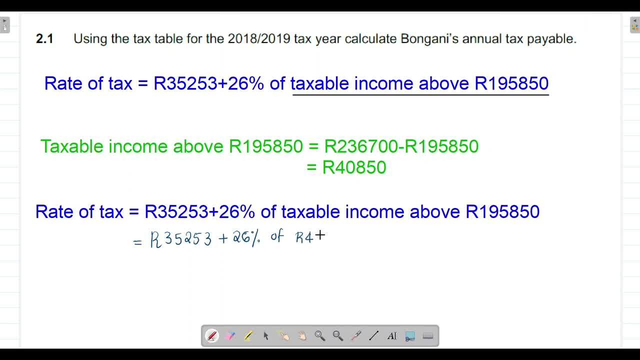 That taxable income. we found that it was $40,850,. okay, And guys, remember I said that when you see that off, it means that we need to multiply, right? So it's the same as just saying $35,253 plus 26% is the same as just saying 26 divided by 100, multiplied by that $40,850. 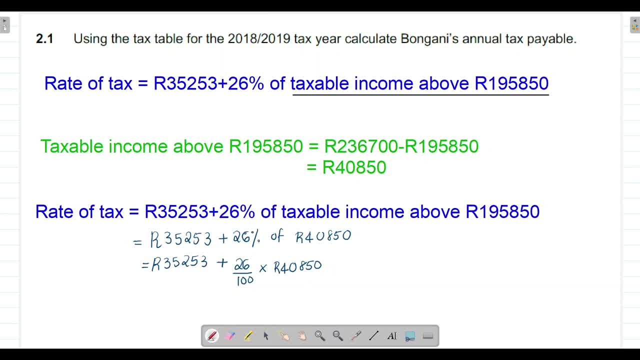 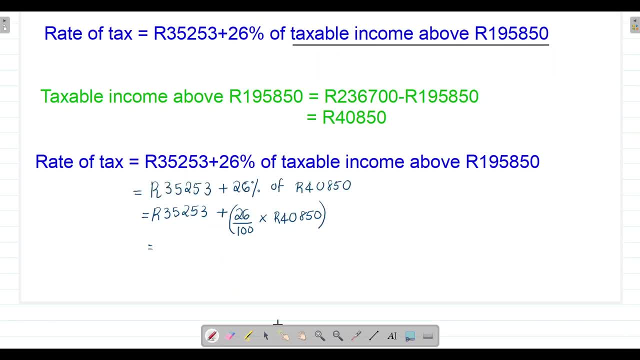 Guys, then here, when I mentioned, when you're doing mathematical literacy, guys, you need to basically show all the bits and pieces. How did you basically get to your answer? okay, So show all the bits and pieces. So it's going to be $35,253 plus what is 226 divided. 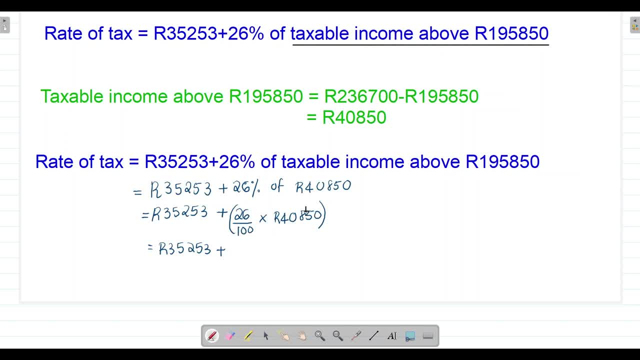 by 100, multiplied by $40,850, okay, You will get that it's actually $10,000, 621.. And all that you need to do now you need to add these two amounts together, right? And when you punch it into your calculator, you'll get $45,874, okay. 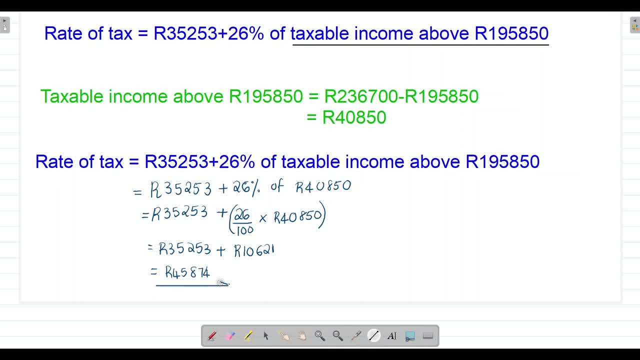 So that is the total amount that he basically has to pay for tax when we basically look at his taxable income. However, guys, this is where you guys need to basically understand that we are not done. okay, Why are we not done? Because we are given the rebates table. 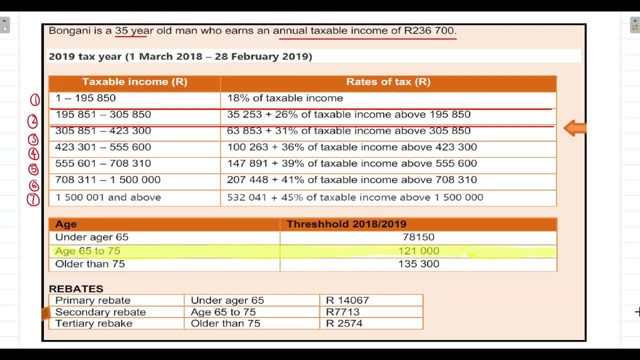 okay, The rebates, basically tells us that, right, we need to basically subtract, okay, the rebates, okay, from this rate of tax that we've basically calculated to get the total that he actually needs to pay for tax. okay, So, in this case, because we are told that Obongani is 35, 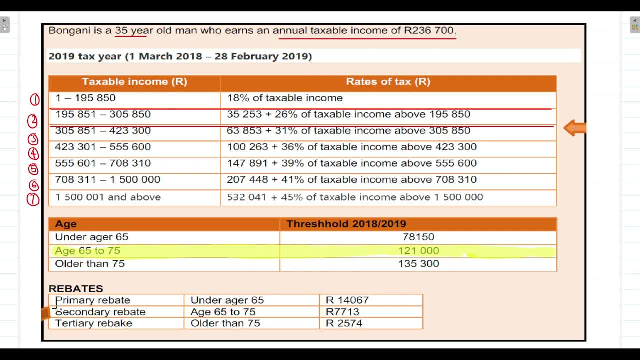 years old. right, we know that. he just qualifies to just get the primary rebate. He doesn't qualify to get the secondary rebate. He doesn't qualify to get the tertiary rebate, He only qualifies to get the primary rebate. So basically what that means is: 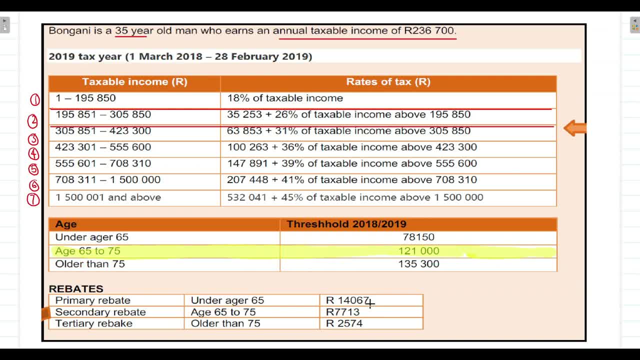 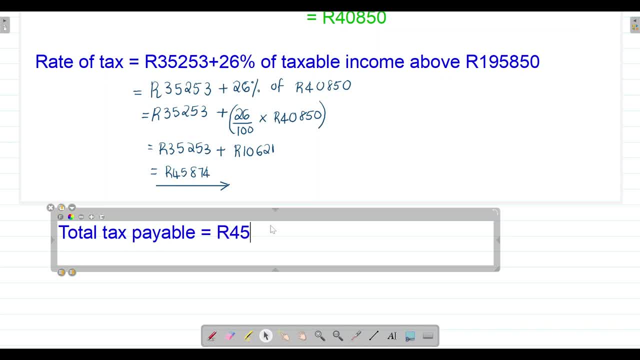 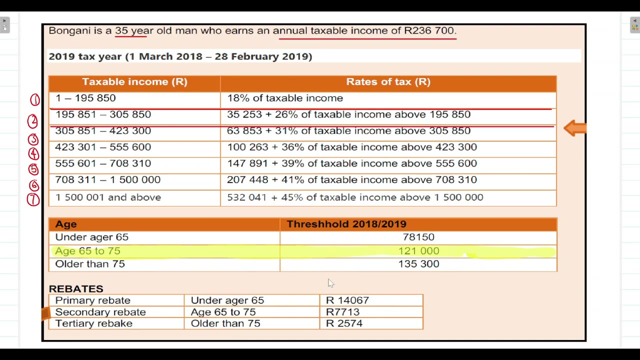 that from this rate of tax that we've basically calculated now, okay, the total tax that will be payable right will be this: $45,874 minus the rebate. okay, And which rebate does he basically qualify for? Here we can see that he only qualifies for the primary rebate, because I 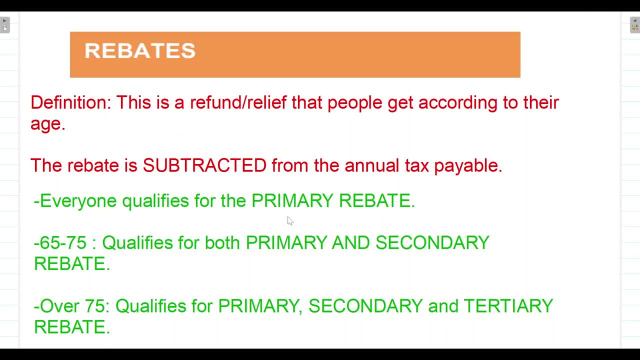 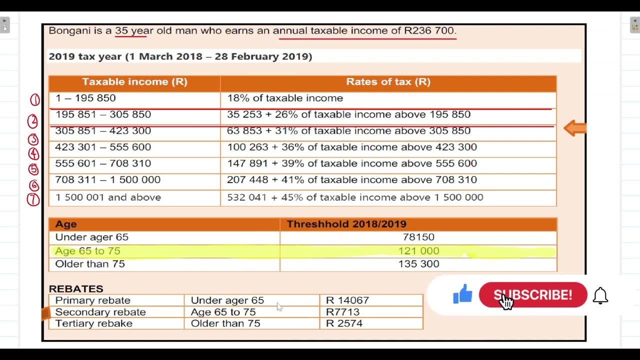 explained that everyone qualifies for the primary rebate. okay, And even the table shows you that if you are basically under the age of 65, right, okay, you qualify for the primary rebate. So, but then in this case, Obongani only qualifies for the primary rebate. So that means that we basically 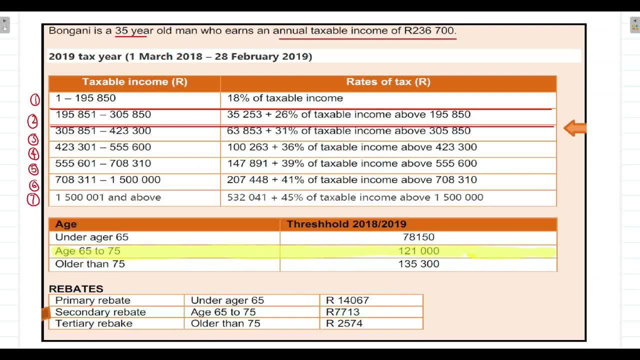 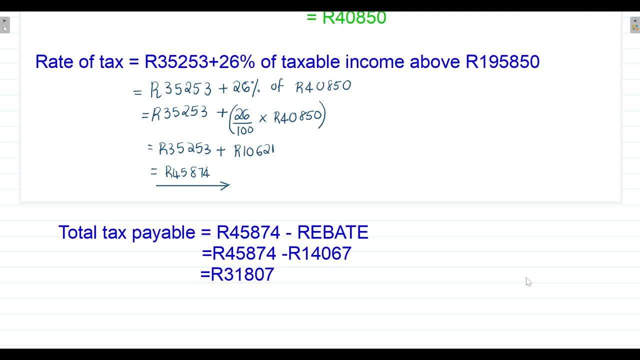 need to subtract that $14,067, right, okay, So basically how much, or the amount that Obongani will have to pay towards his tax. right after we've basically subtracted, the rebate is actually $31,807, okay, So just quickly. 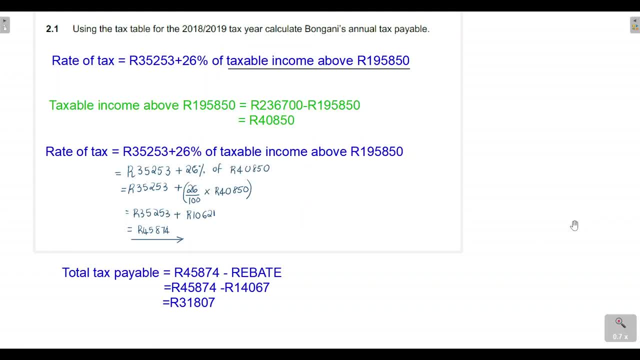 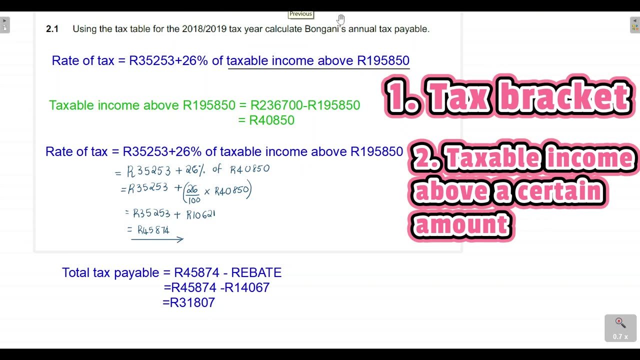 when it comes to calculating the total tax payable, you need to first determine the tax bracket that his income falls in right And then you need to basically determine how much of that taxable income Is above a particular amount, based on the formula that you are given from the tax bracket that his 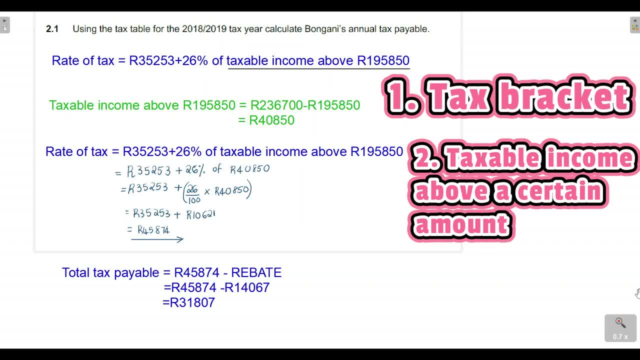 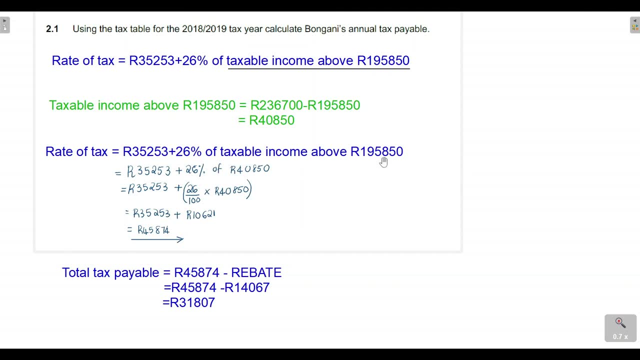 salary falls in right, And then, once you've basically determined that, you now need to substitute that amount into your formula, right? Because now, in this case, we found that $40,850 of his taxable income is actually above $195,850,. okay, Then, from there, all we needed to do was 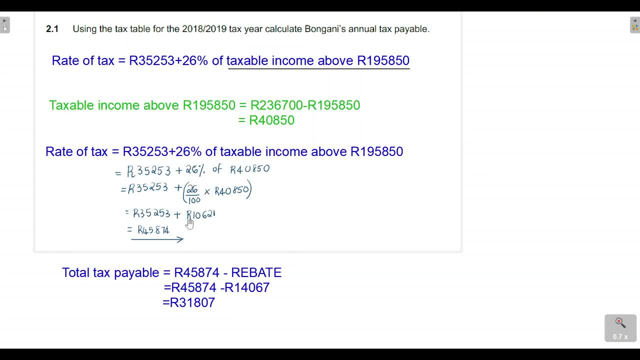 then now multiply that amount by 26%, and we did that, okay. And when we did that, we found that now it is 26% of his taxable income is actually $10,621,. all right, Then, from there, we just added that. 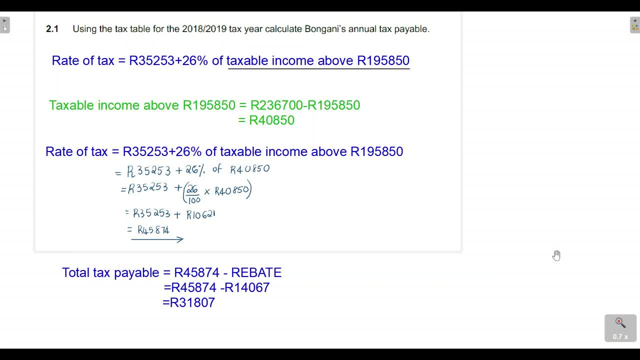 to get only what is his rate of tax? what is his rate of tax based on the tax bracket that he falls in? okay, We are not done. We still need to subtract the rebate. And what helps us determine that is his age? 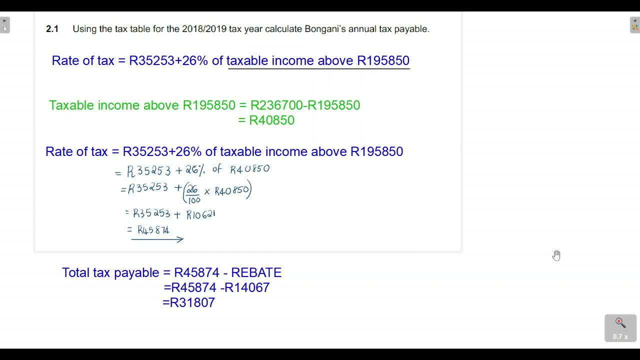 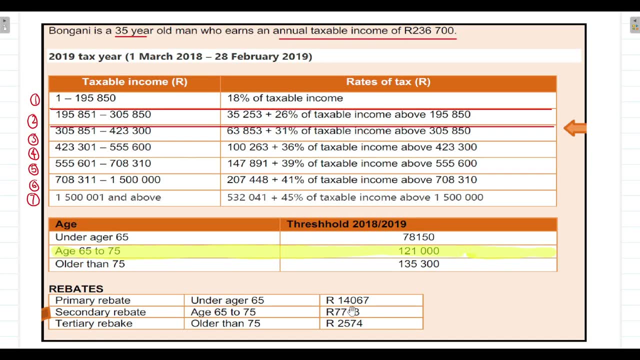 In this case, because Wang An is 35 years old, we know he only just qualifies to get the primary rebate. Therefore, we subtract that primary rebate of $14,067.. And in this case, when you subtract that, you got $31,807.. Please note. okay, like I mentioned, I think this table will. 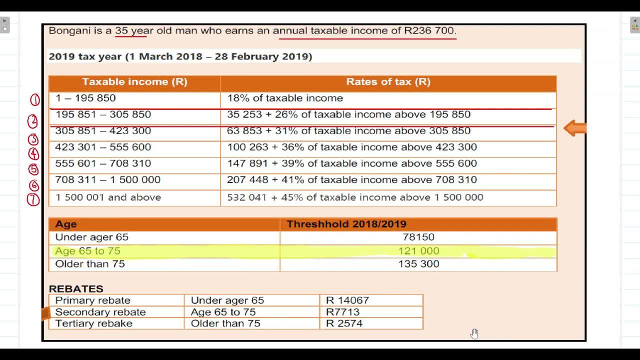 basically create a lot of confusion, especially if you're a learner that doesn't know what you're doing. You'll just think: let's say, for example, they gave us like a 65-year-old, okay, If let's say Ubo Ngani was 65 years old, right, We would basically need to minus the primary rebate as well. 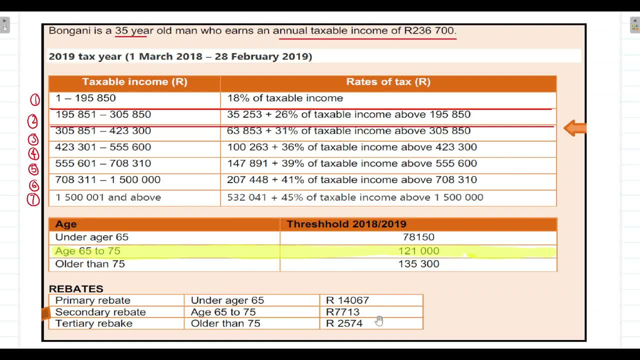 as the secondary rebate. okay, Because for you to qualify to get the secondary rebate, you need to be between the ages of 65 years to 75 years. Then if Ubo Ngani was 65 years old, we'd have to minus actually both of these rebates. okay, All right. So I hope you guys understand that point. 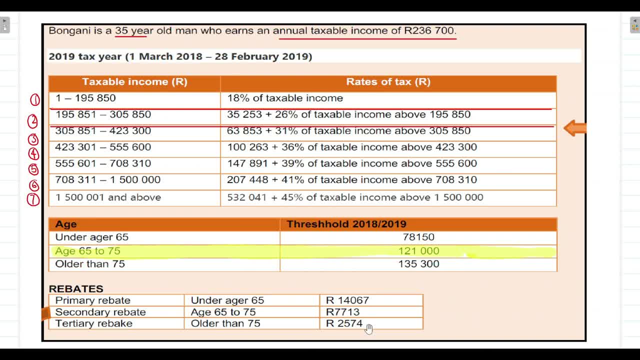 because I think that's where most learners are going to be. So I hope you guys understand that point because I think that's where most learners are going to be. So I hope you guys understand that will get this incorrect, because this table can be a bit confusing, especially if you do not know. 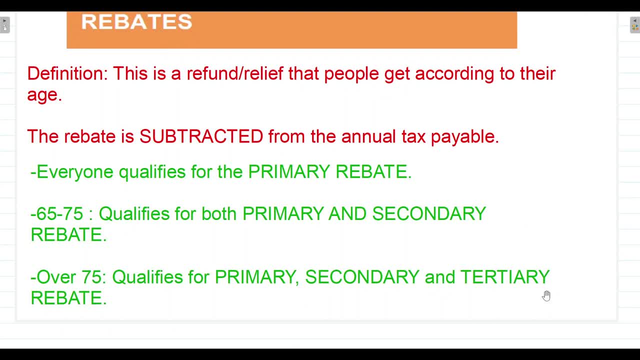 what I just explained to you guys here, that everyone qualifies for the primary rebate, right. And then if you're between the ages of 65 to 75 years old, you qualify for both the primary and the secondary rebates, And if you're over 75 years old, you qualify for the primary rebates. 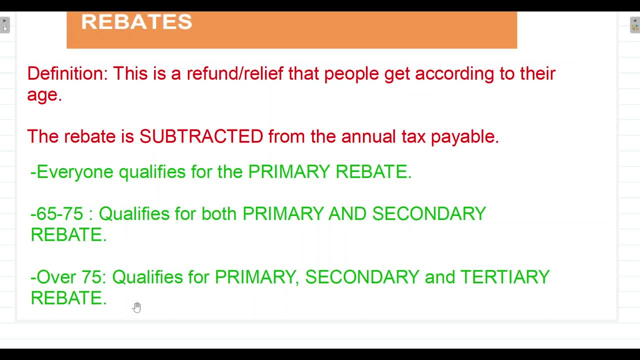 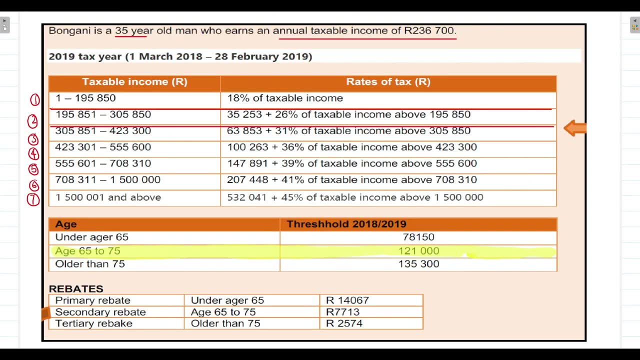 you qualify for the secondary rebates and you also qualify for the tertiary rebates. okay, That is very important guys. You need to understand that point because if you don't, you'll get the last part of this calculation incorrect. That is a super tip for your exams. 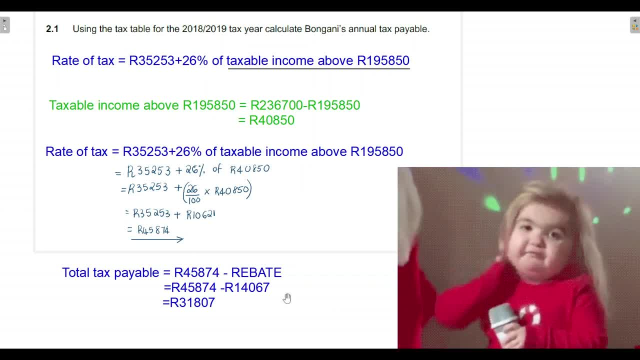 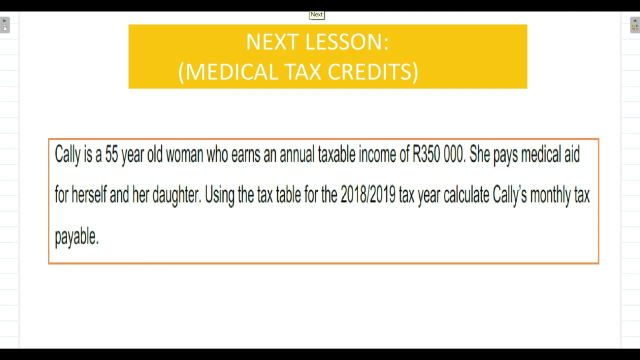 It doesn't get any better than that. okay, All right, So I'm going to end this video tutorial here, guys, right In the next video tutorial, we will be discussing what happens now if we add medical aid into the scenario. right, We've got rebates, we've got medical. 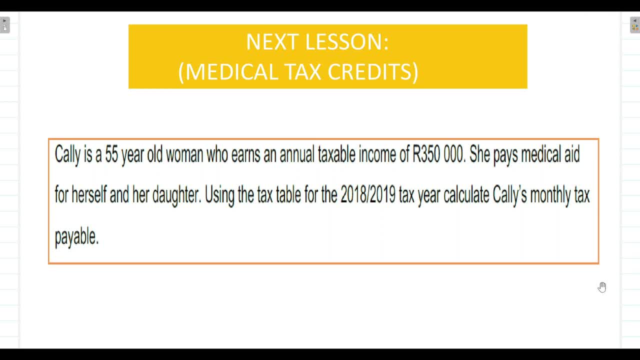 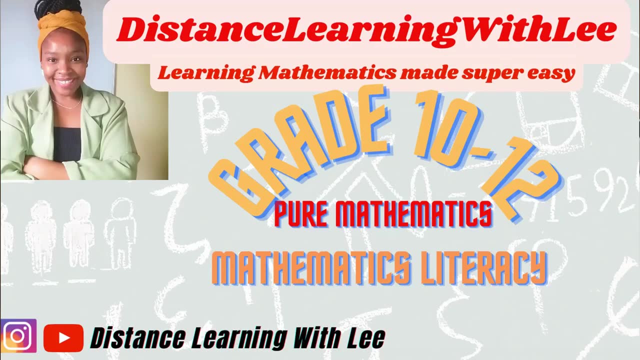 what happens. How do we calculate the total tax that Carly will have to pay? okay, So please make sure that you watch the next lesson where I'm going to be explaining that to you guys. That is it, guys, And I'll see you guys on my next upload. Distance Learning with Leigh. 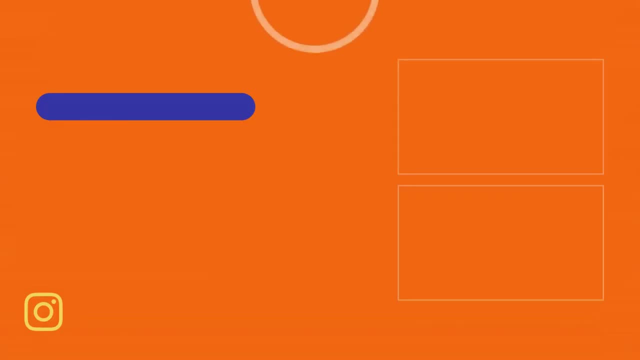 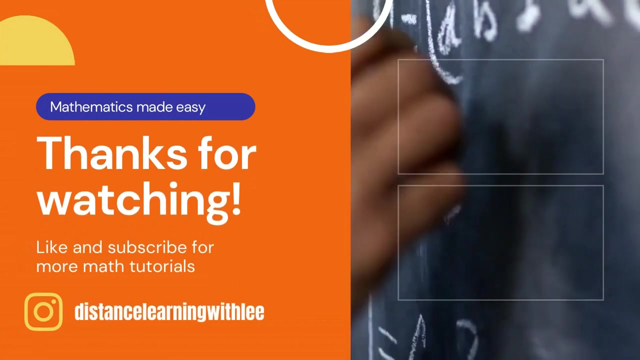 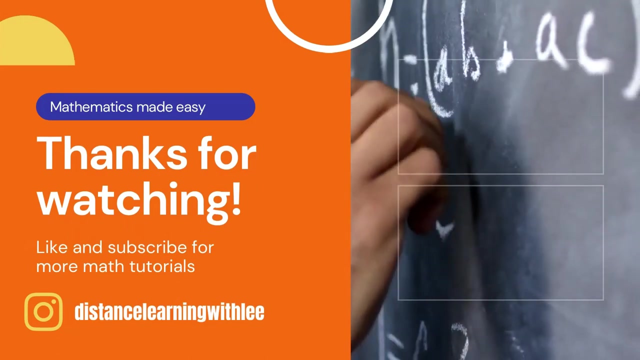 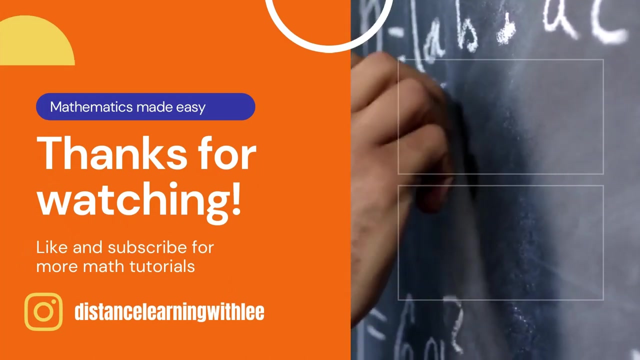 where I make learning mathematics super easy. Bye, Transcription by CastingWords.